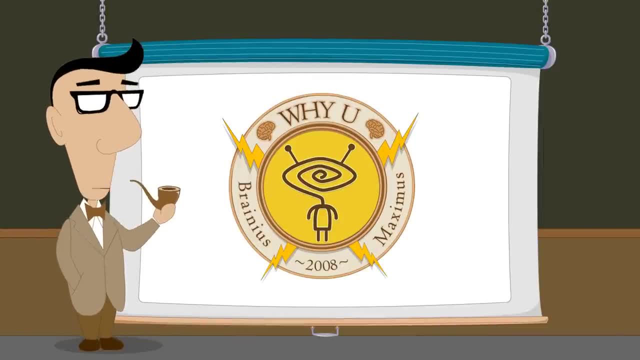 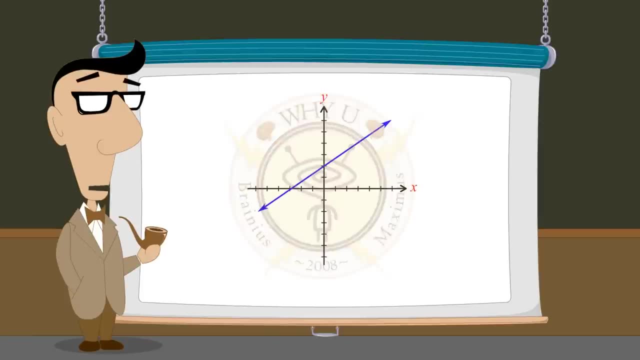 Hello, I'm Professor Von Schmohawk and welcome to Why U. In the last several lectures we introduced several forms of linear equations whose graphs are lines in the x-y plane. In this chapter we will use linear equations to solve some real-world problems. 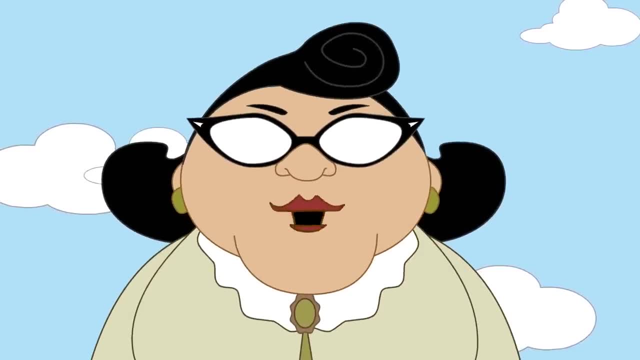 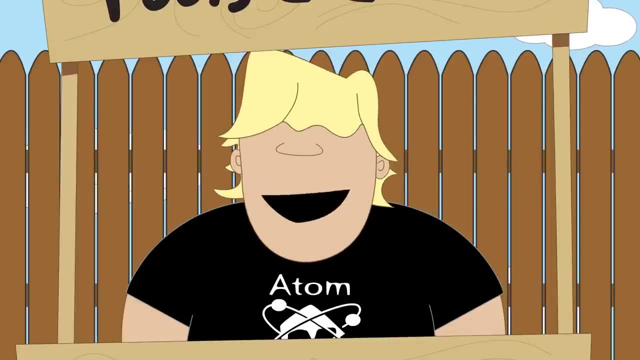 Why? hello Hulk, I'm so happy to see that you are gainfully employed this summer. I was looking for someone to drain my pool tomorrow. Uh sure, Professor Atheline, but I'm supposed to clean Mr Squeegeopolis' pool tomorrow. 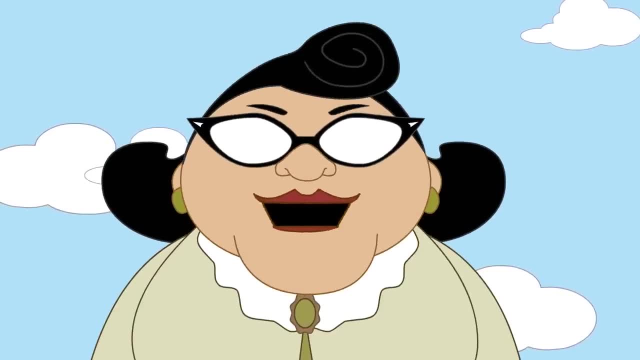 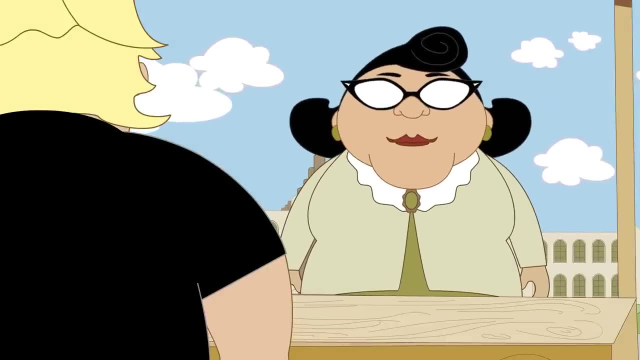 Well, I'm sorry, Hulk, but I need it drained by 8 pm. tomorrow. I'm having some very important guests over and the pool must be completely empty by the time they arrive. Okay, Professor, I'll figure something out. 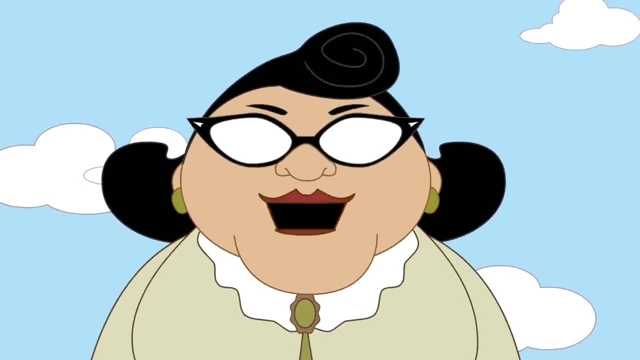 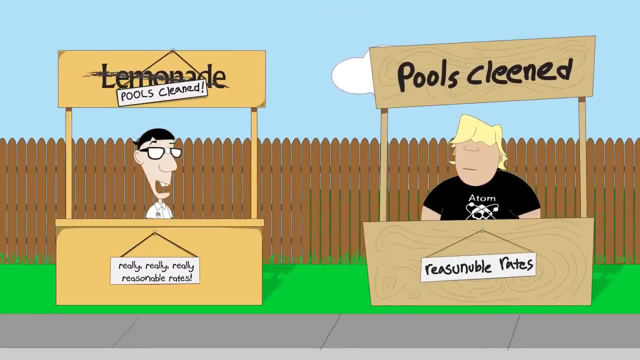 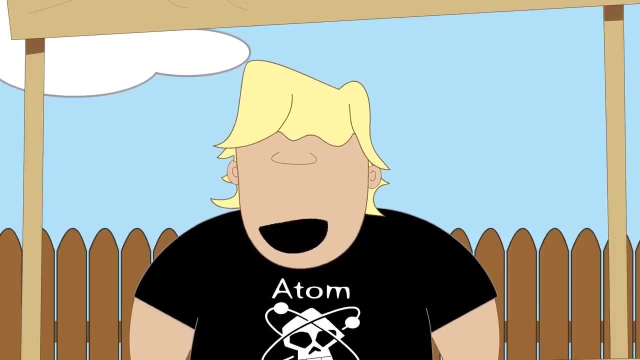 Oh, Hulk, you're such a resourceful young man I knew I could count on you. Ahem, What's the matter, Hulk? Have you perhaps encountered a small resource scheduling problem? Okay, Geekman, How much is this gonna cost me? 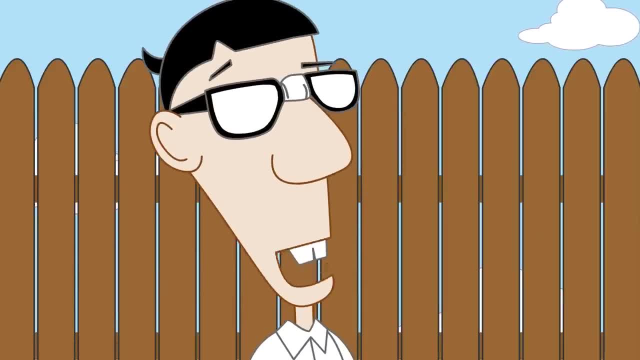 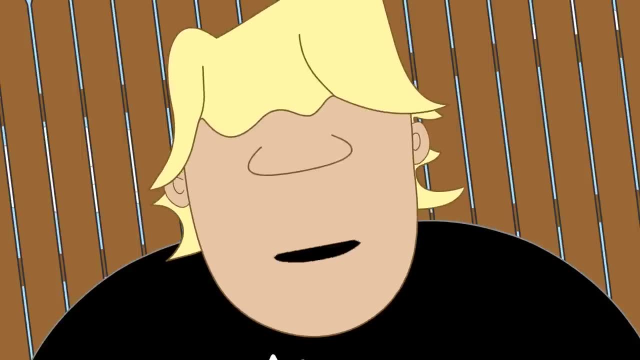 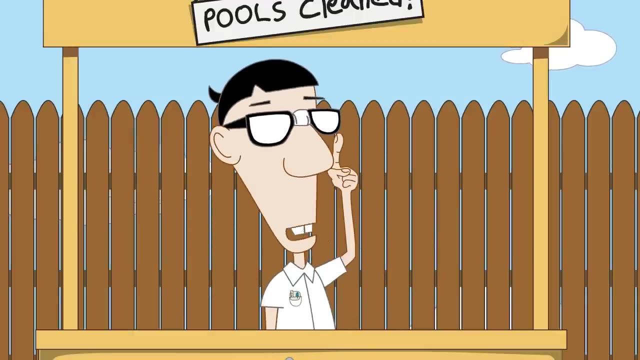 Well, my normal short notice subcontracting fee is $50 an hour, but I'm running a special today, Only 49 buckaroonies an hour. Yeah Well, I'm running a special today on knuckle sandwiches. Perhaps I didn't mention that you're eligible for the double-extra-special-very-best-buddy rate of $3 an hour. 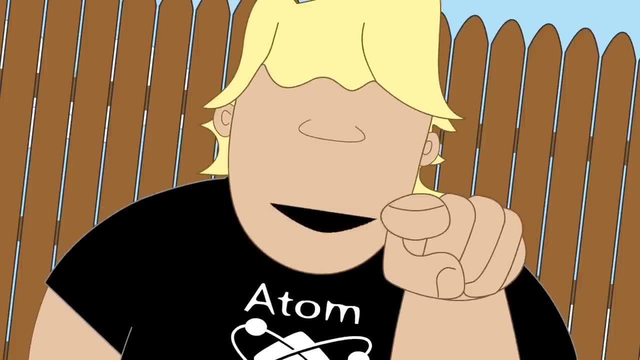 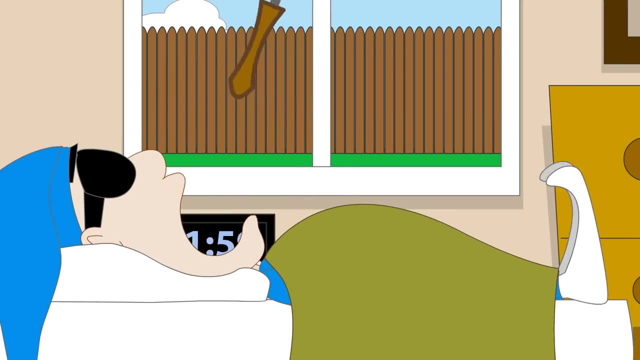 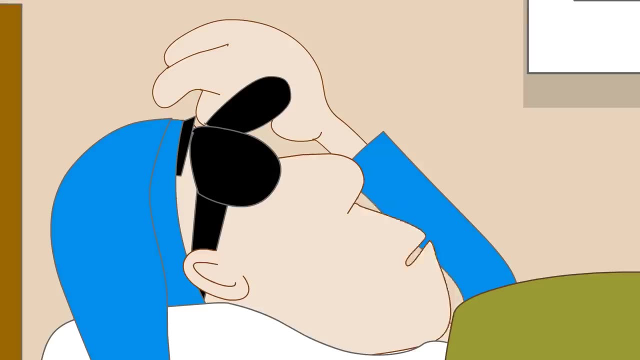 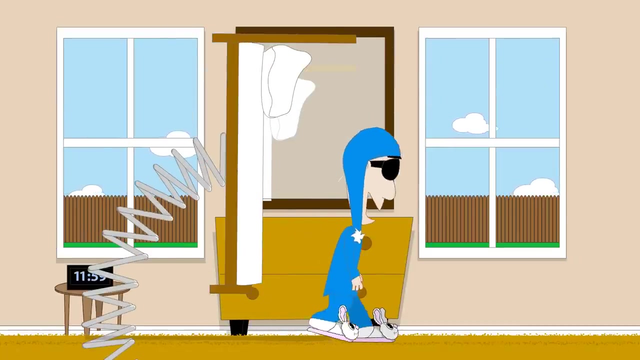 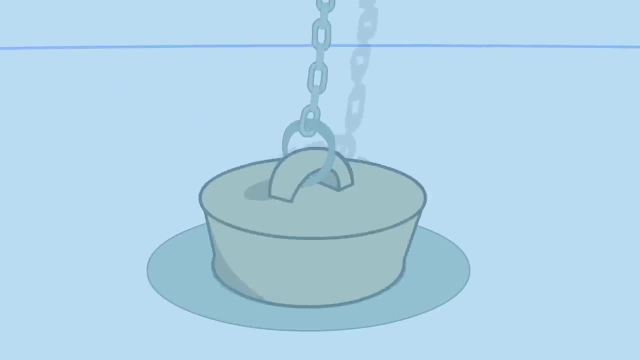 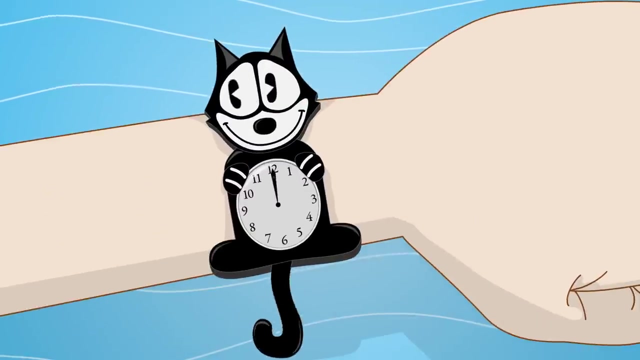 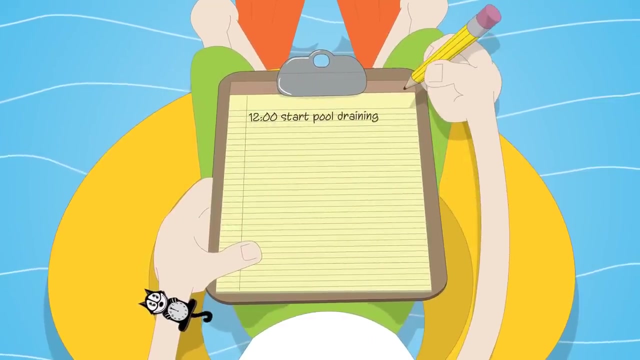 Well, just make sure you have that pool empty by 8 pm tomorrow. Yes, sir, Mr Booshmasher, Grats, it's almost noon, I'd better get crackin'. I know, Start pool draining at 12 noon. 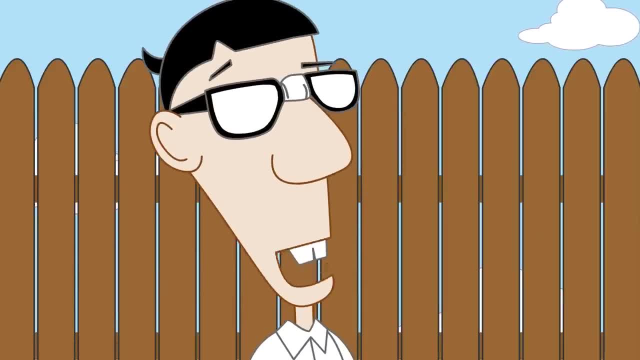 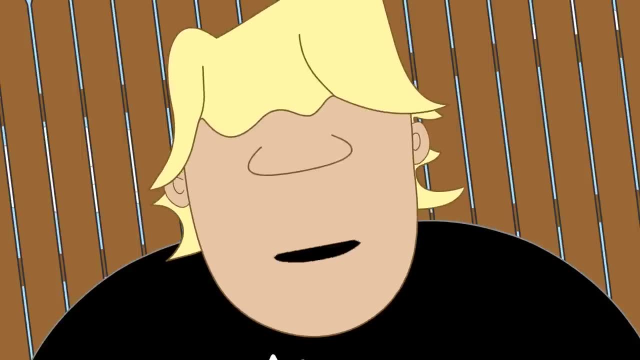 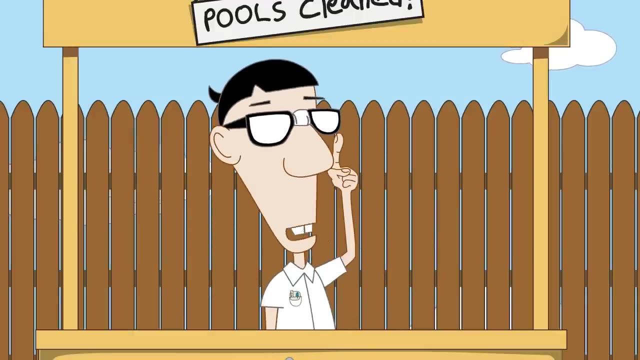 Well, my normal short notice subcontracting fee is $50 an hour, but I'm running a special today, Only 49 buckaroonies an hour. Yeah Well, I'm running a special today on knuckle sandwiches. Perhaps I didn't mention that you're eligible for the double-extra-special-very-best-buddy rate of $3 an hour. 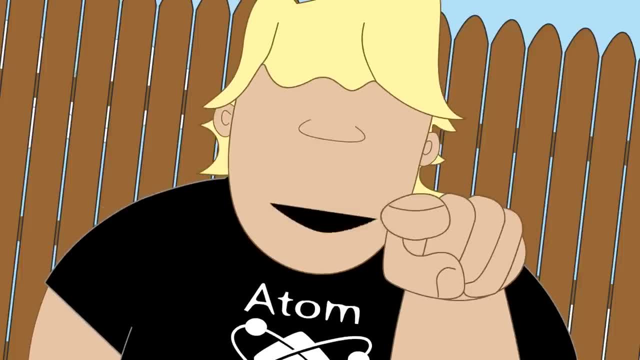 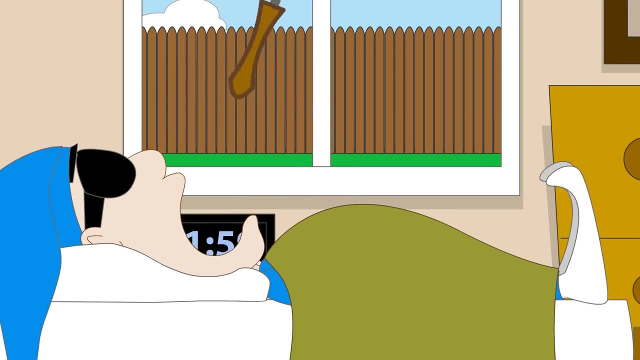 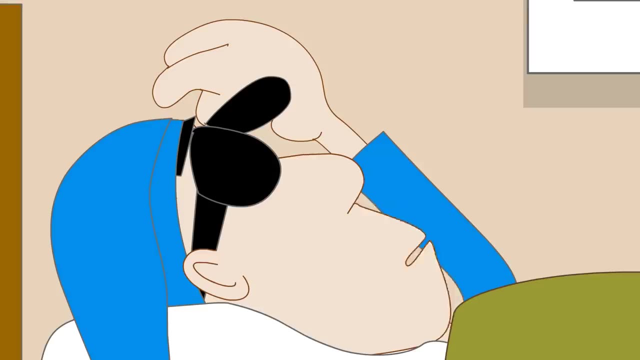 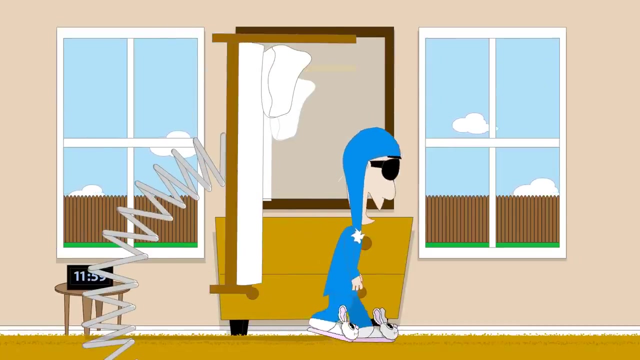 Well, just make sure you have that pool empty by 8 pm tomorrow. Yes, sir, Mr Booshmasher, Grats, it's almost noon, I'd better get crackin'. I want a drink too. 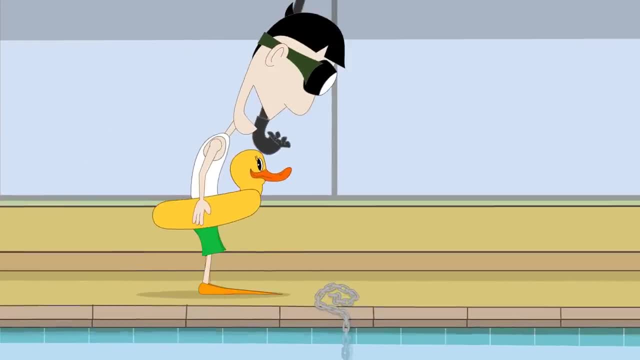 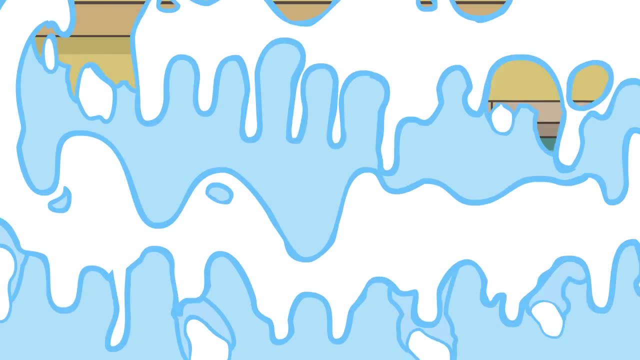 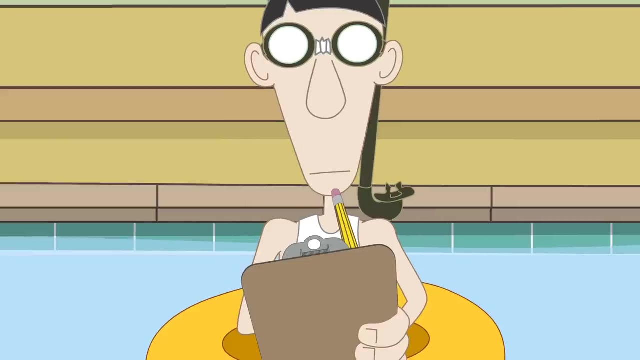 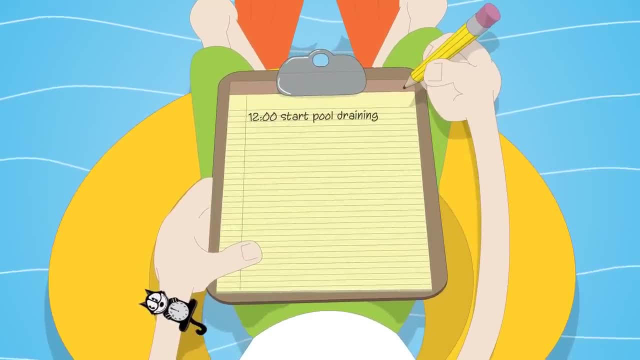 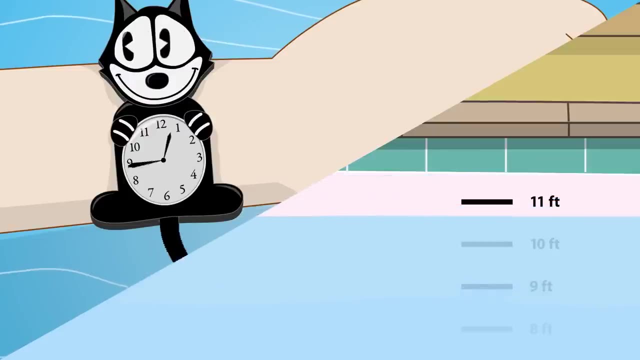 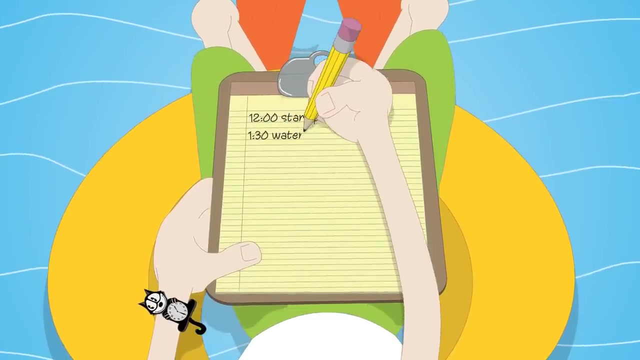 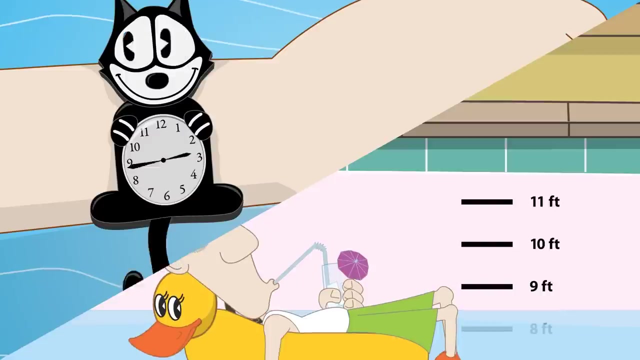 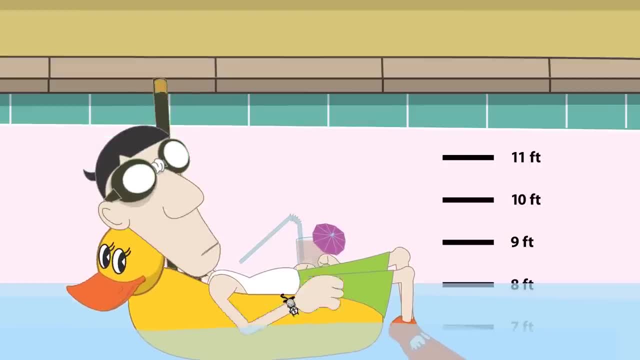 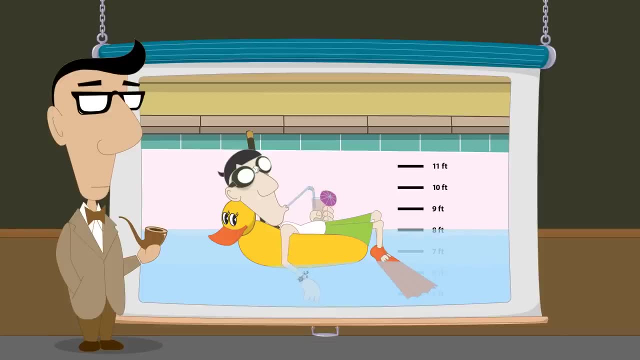 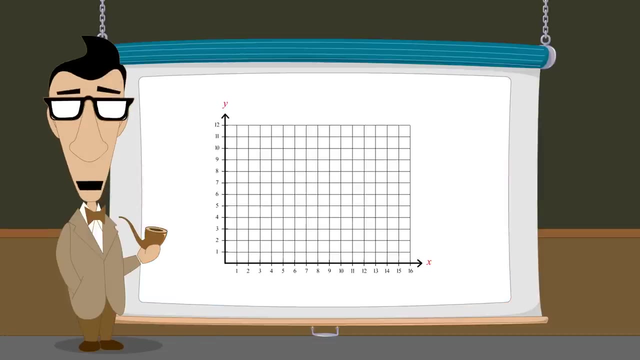 Yikes, this pool better be empty by 8 pm. Well, it looks like Ace Algebra student AV Geekman may be in hot water. Will the pool be empty by 8 pm? If we graph the water depth versus time, 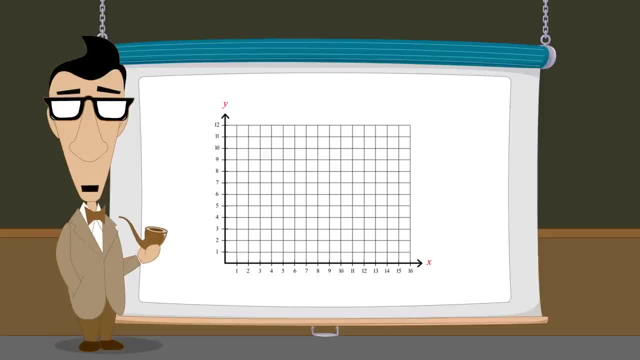 we might be able to figure out how long it will take for the pool to completely drain. We will plot the amount of time since the drain was first opened at noon on the horizontal axis and water depth on the vertical axis. We know that at 1.30, one and a half hours after the drain was opened, the water level was 10 feet. 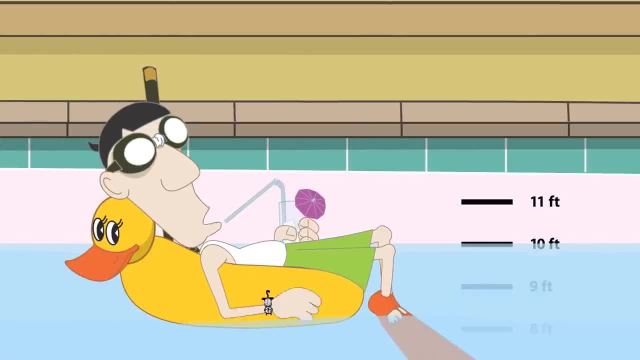 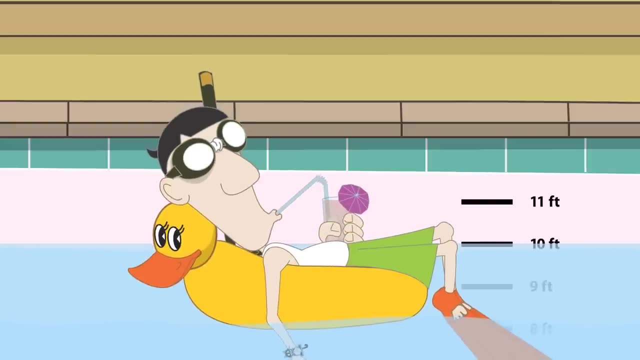 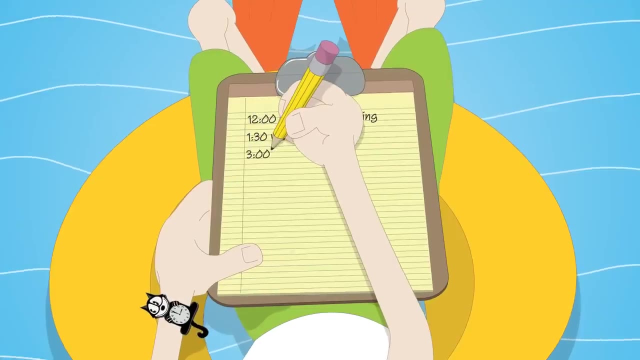 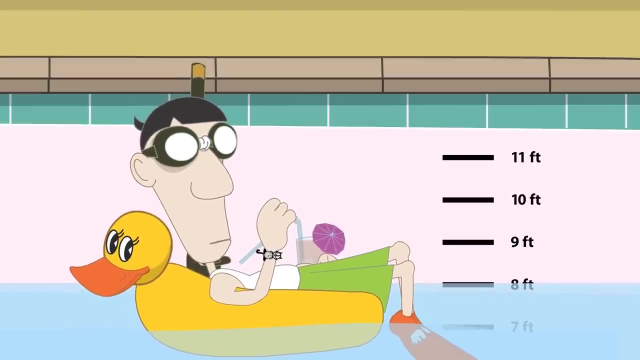 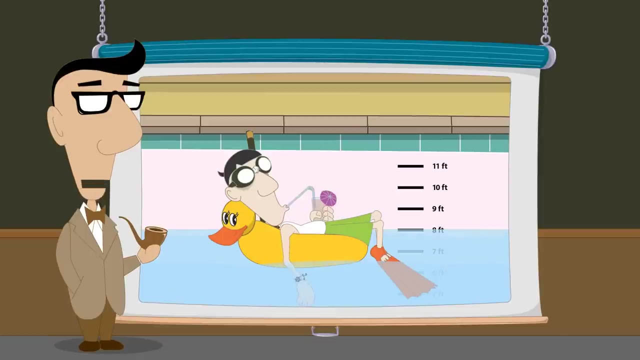 Hmm, it's 1.30, and the water level is 10 feet. Hmm, 3 o'clock and the water level is 8 feet. Yikes, this pool better be empty by 8 pm. Well, it looks like Ace Algebra student AV Geekman may be in hot water. 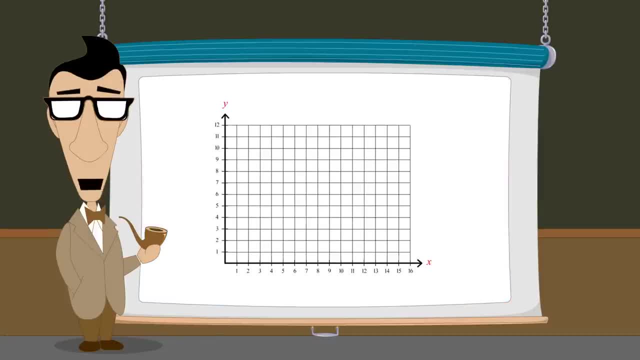 Will the pool be empty by 8 pm? If we graph the water depth versus time, we might be able to figure out how long it will take for the pool to completely drain. We will plot the amount of time since the drain was first opened at noon on the horizontal axis. 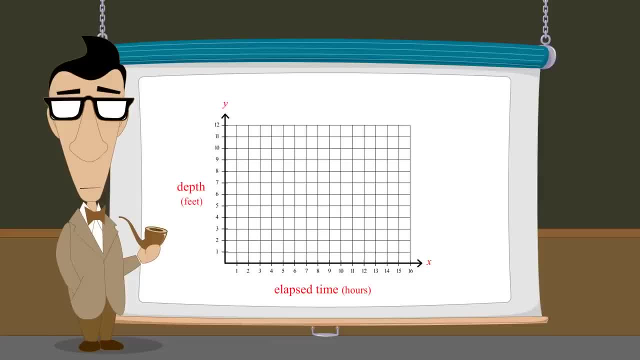 and water depth on the vertical axis. We know that at 1.30, one and a half hours after the drain was opened, the water level was 10 feet, and at 3 o'clock, after three hours of draining, the water level was 8 feet. 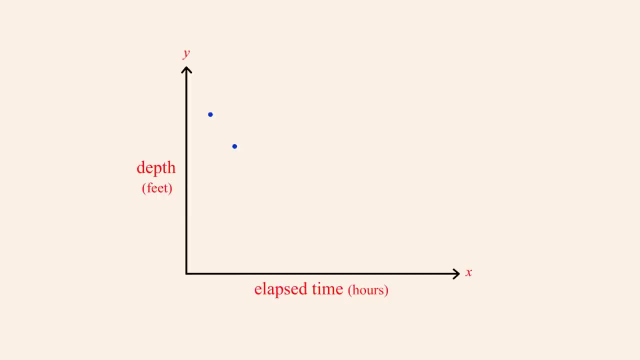 However, there is one problem: With only two data points, it is impossible to determine whether the water level is dropping by the same amount every hour, or if the water level drops more quickly as time goes on, or if the water level drops more quickly as time goes on. 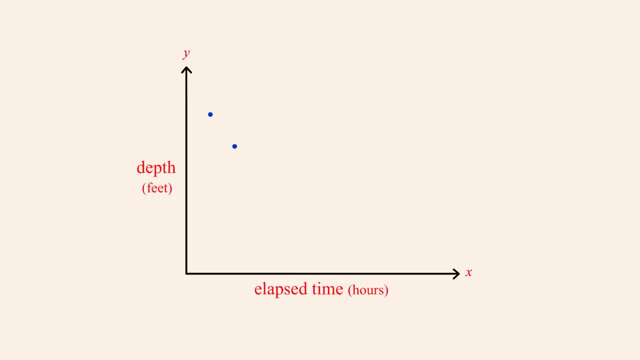 or perhaps if the water level drops more slowly with increasing time? or perhaps if the water level drops more slowly with increasing time. Taking one additional measurement, a third time, would allow us to determine which scenario more accurately represents the water level as a function of time. 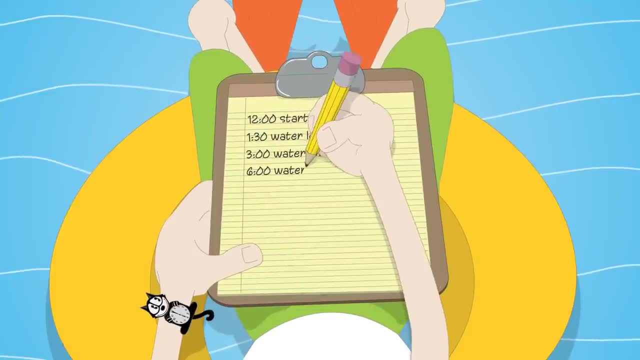 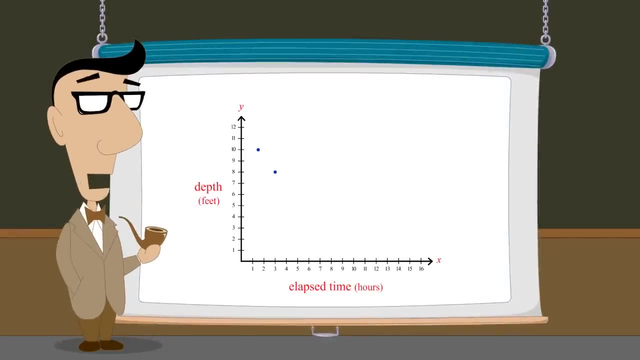 Dang. it's 6 o'clock already And we still have four feet to go. We can now add a third data point to our graph of water depth versus elapsed time, since AV has determined that after six hours the water depth is four feet. 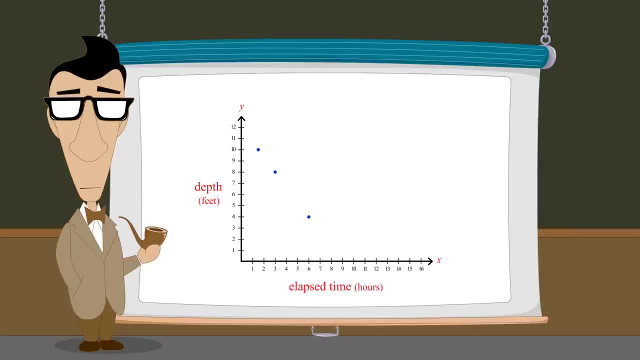 It looks like these three points all fall on a line, so maybe the function we are graphing is linear. We can verify this mathematically by calculating the slopes of the line segments connecting the first and second points and the second and third points, If the slopes of both segments are the same. 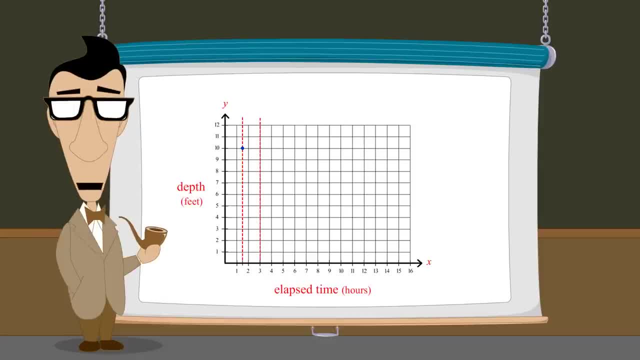 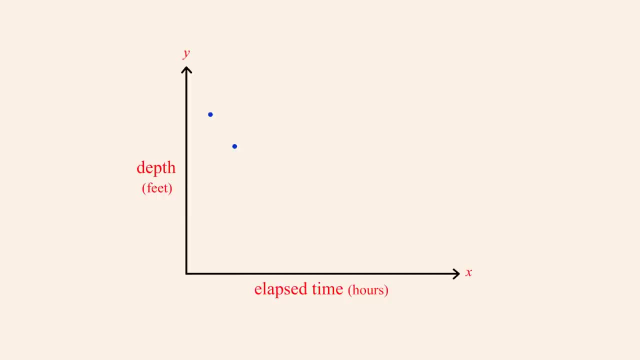 and at 3 o'clock, after three hours of draining, the water level was 8 feet. However, there is one problem With only two data points: it is impossible to determine whether the water level is dropping by the same amount every hour. 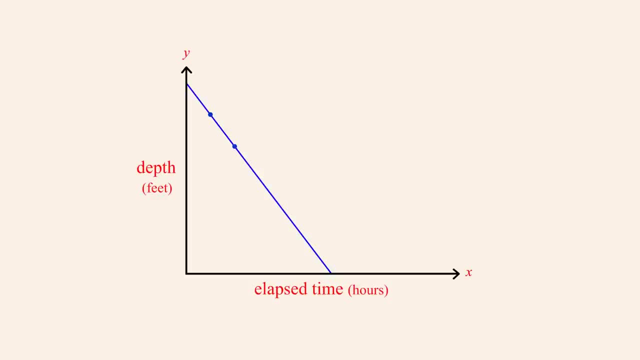 or if the water level drops more quickly as time goes on, or if the water level drops more quickly as time goes on, or perhaps if the water level drops more slowly with increasing time, or perhaps if the water level drops more slowly with increasing time. 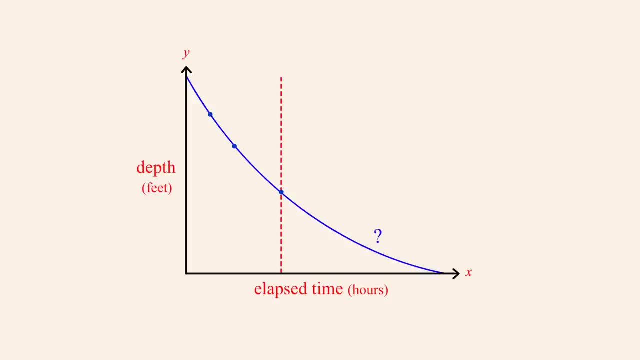 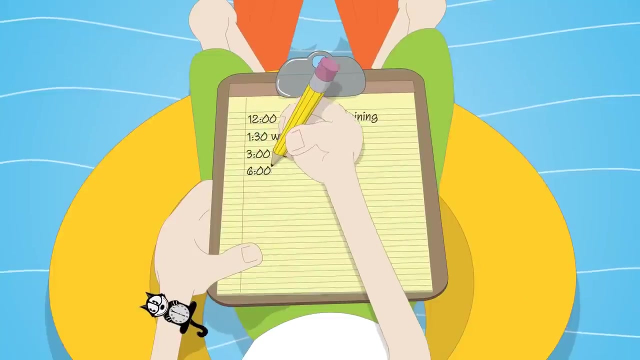 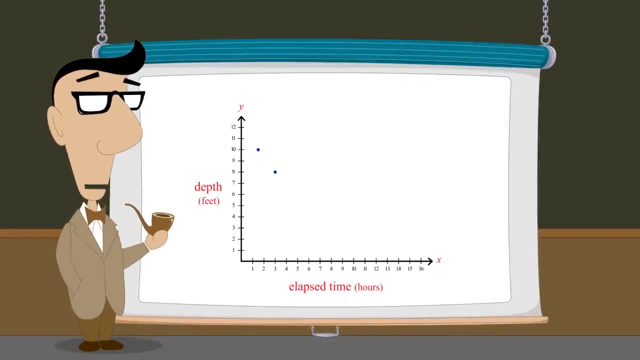 Taking one additional measurement, a third time, would allow us to determine which scenario more accurately represents the water level as a function of time Dang. it's 6 o'clock already And we still have four feet to go. We can now add a third data point to our graph of water depth versus elapsed time. 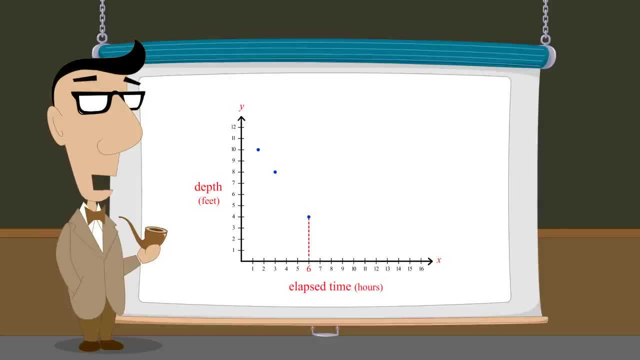 since AV has determined that after six hours the water depth is four feet. It looks like these three points all fall on a line, so maybe the function we are graphing is linear. We can verify this mathematically by calculating the slopes of the line segments. 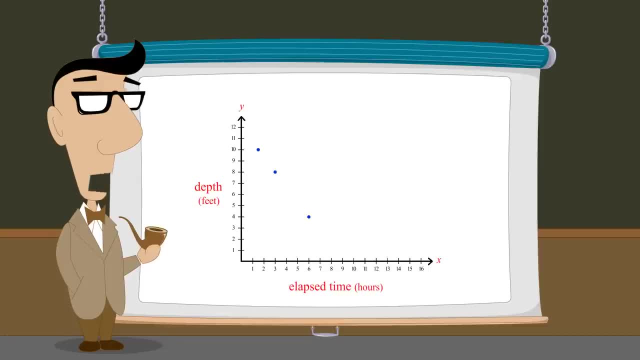 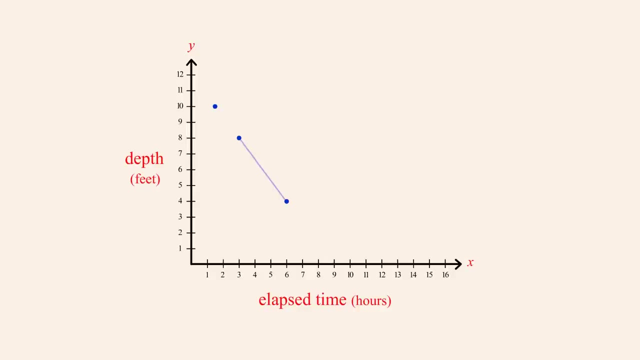 connecting the first and second points and the second and third points. If the slopes of both segments are the same, then all three points must lie on the same line. As we saw in the chapter on slope, we can calculate the slope of a line which passes through two points. 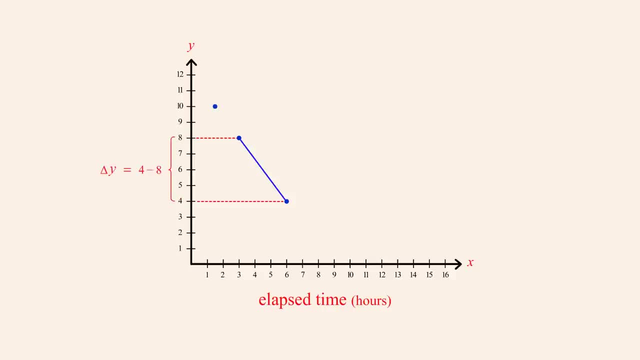 as the difference in the point's y-coordinates, delta y, divided by the difference in their x-coordinates, delta x. Dividing delta y by delta x, we get negative four over three or a slope of negative four thirds. Now let's calculate the slope of the other line segment. 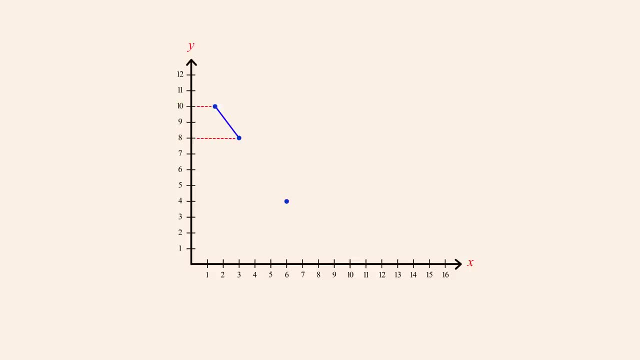 Once again, we take the difference in the y-coordinates- delta y, and the difference in the x-coordinates- delta x. Dividing delta y by delta x, we get negative two over three halves. We can simplify this complex fraction by dividing negative two by three halves. 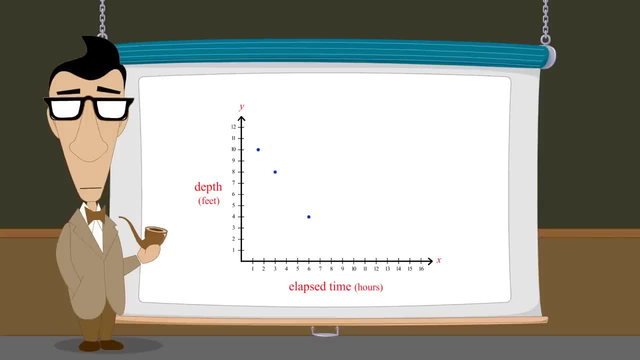 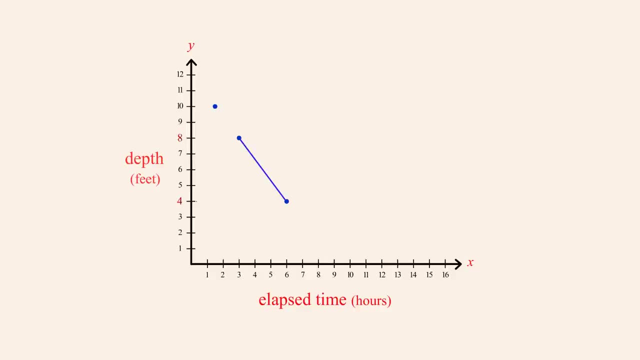 then all three points must lie on the same line. As we saw in the chapter on slope, we can calculate the slope of a line which passes through two points as the difference in the point's y-coordinates- delta y- divided by the difference in their x-coordinates- delta x. 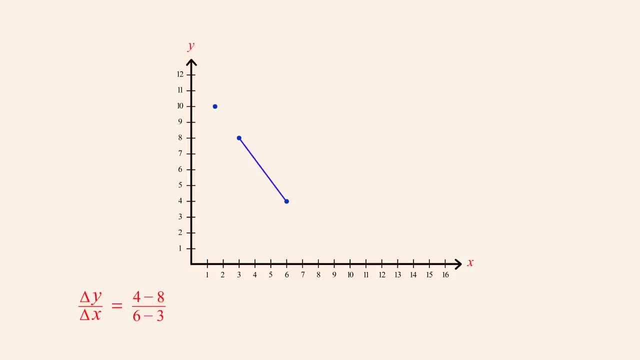 Dividing delta y by delta x, we get negative four over three, or a slope of negative four thirds. Now let's calculate the slope of the other line segment Once again. we take the difference in the y-coordinates- delta y and the difference in the x-coordinates- delta x. 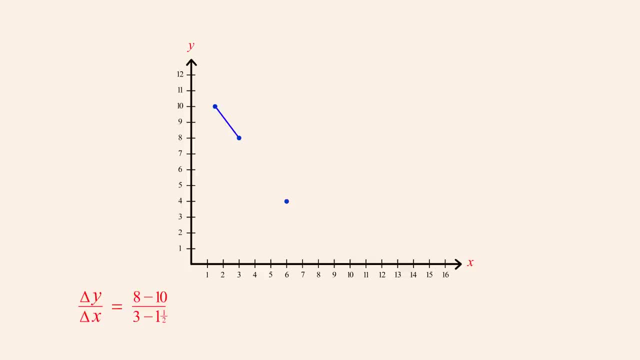 Dividing delta y by delta x, we get negative two over three halves. We can simplify this complex fraction by dividing negative two by three halves. This is the same as multiplying negative two times the reciprocal of three halves, or two thirds. Negative two times two thirds is negative four thirds. 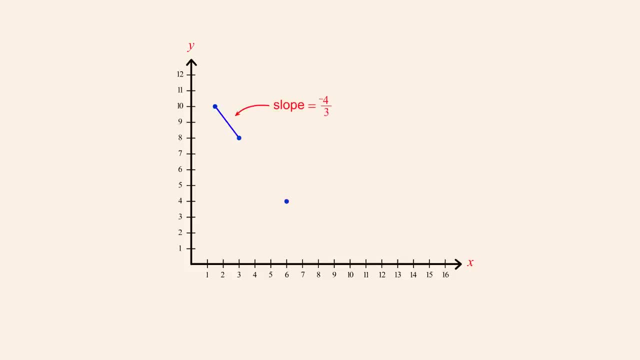 So the slope of this line segment is also negative four thirds. Since the slopes of these two connected line segments are the same, all three points must lie on the same line. We can therefore assume that the water in the pool is draining at a constant rate. 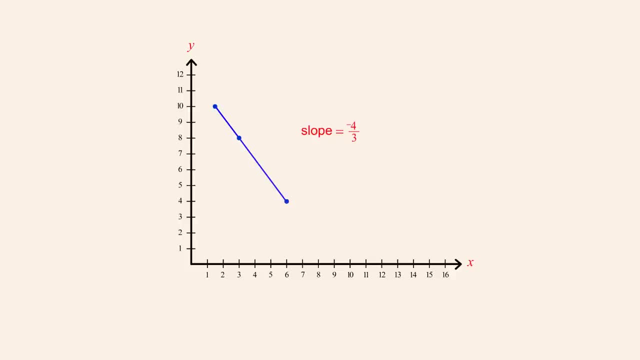 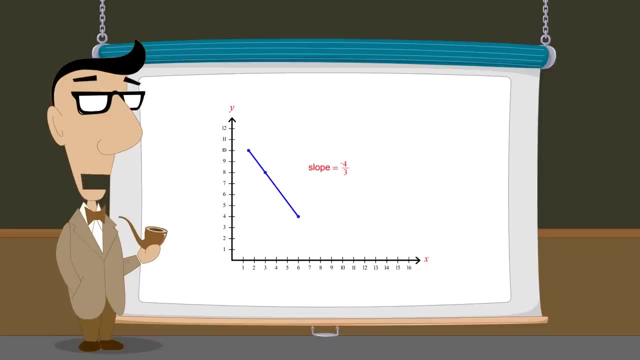 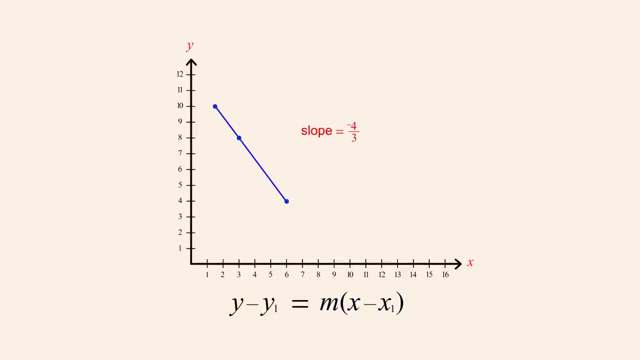 and that the water depth, as a function of time, is linear. Since we know this line's slope and at least one point which falls on the line, we can write the equation for this line using the point slope form If we choose the bottom point, which has coordinate six-four. 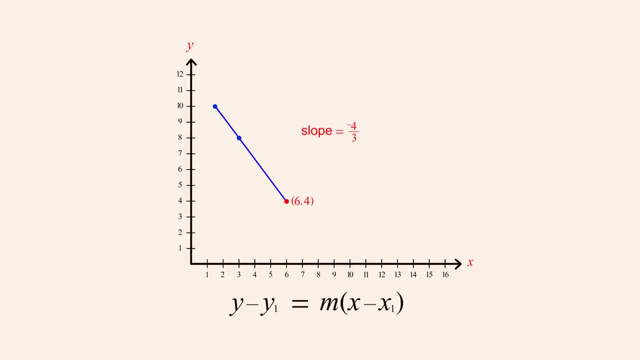 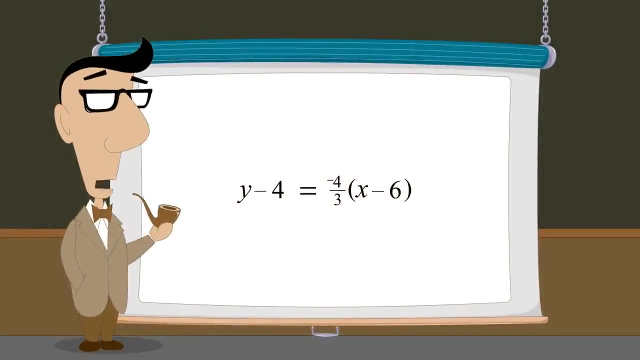 to use as the known point in the point slope formula. then x-one is six, y-one is four and the slope m is negative four thirds. Now that we have an equation which represents water level y as a function of elapsed time, x, we can plug in different values for x. 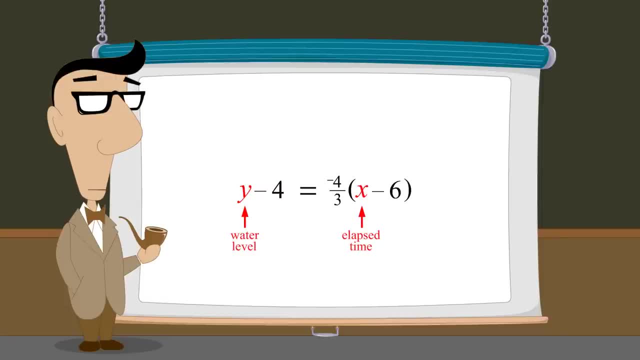 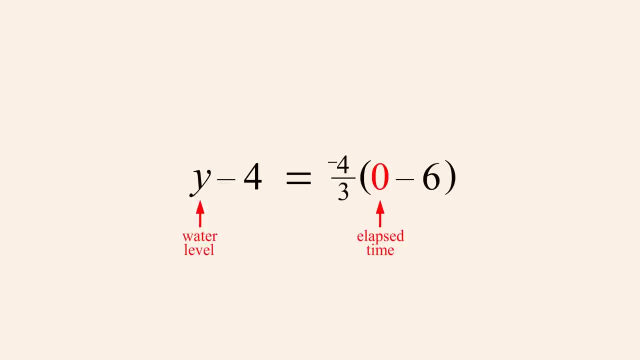 to see what the water level will be at those points in time. For example, an elapsed time x of zero corresponds to the time when the drain was first opened. If we set x to zero, then the resulting value of y will tell us the initial depth of the pool. 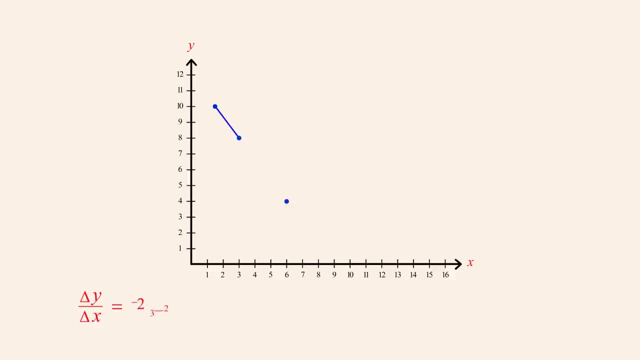 This is the same as multiplying negative two times the reciprocal of three halves, or two thirds. Negative two times two thirds is negative four thirds. So the slope of this line segment is also negative four thirds. Since the slopes of these two connected line segments are the same, 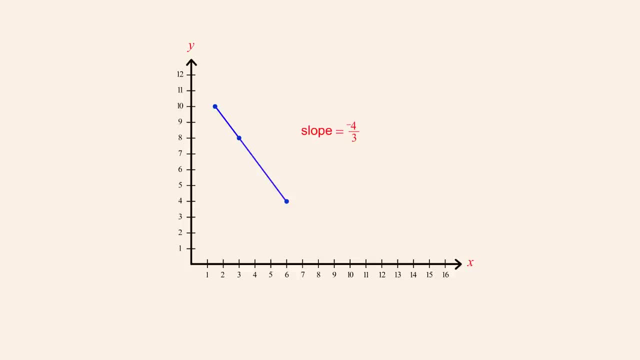 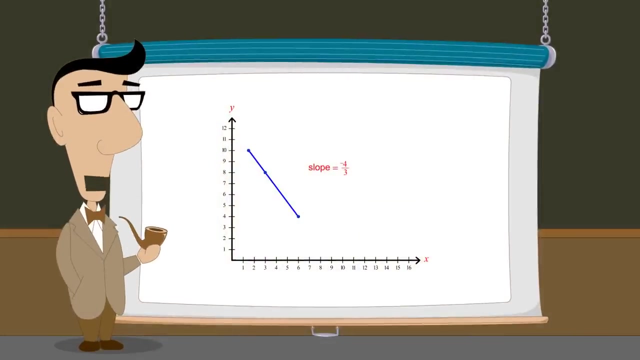 all three points must lie on the same line. We can therefore assume that the water in the pool is draining at a constant rate and that the water depth, as a function of time, is linear, Since we know this line's slope and at least one point which falls on the line. 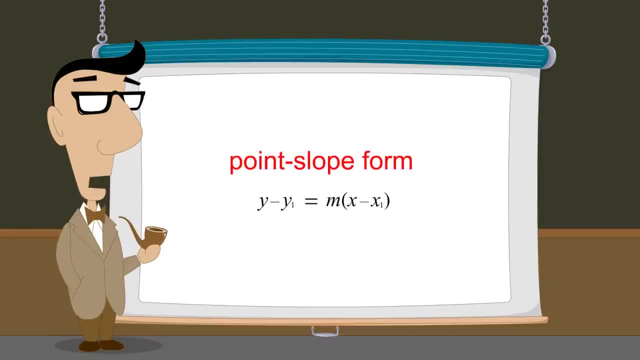 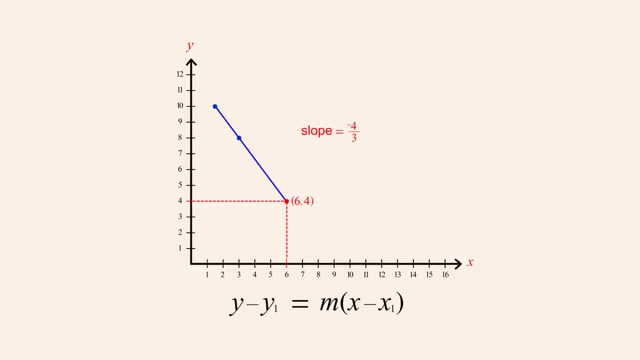 we can write the equation for this line using the point-slope form. If we choose the bottom point, which has coordinate, to use as the known point in the point-slope formula, then x-one is six and y-one is four and the slope m. 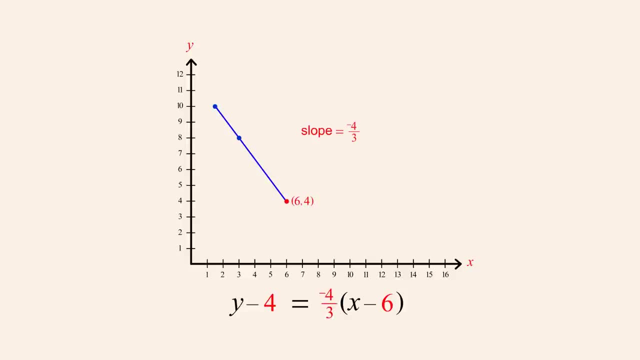 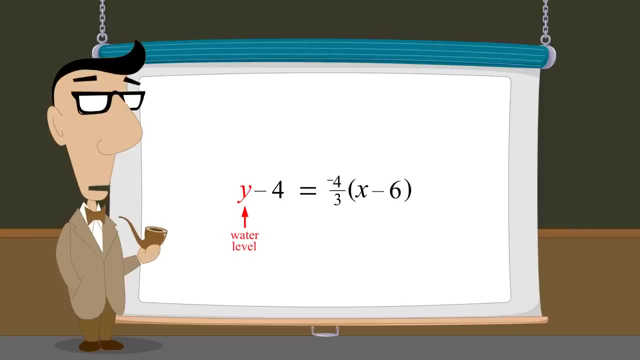 is negative four thirds. Now that we have an equation which represents water level y as a function of elapsed time x, we can plug in different values for x to see what the water level will be at those points in time, For example an elapsed time x. 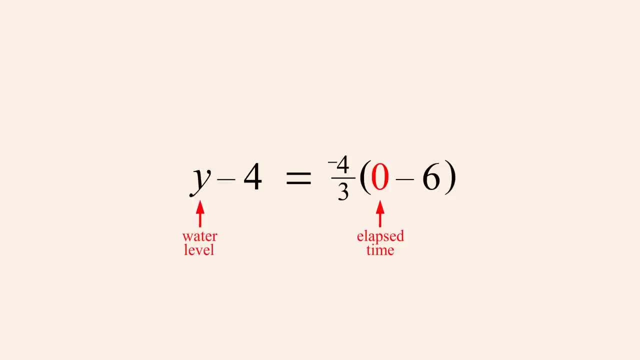 of zero corresponds to the time when the drain was first opened. If we set x to zero, then the resulting value of y will tell us the initial depth of the pool. Completing the arithmetic zero minus six is negative six and negative four thirds times negative six. 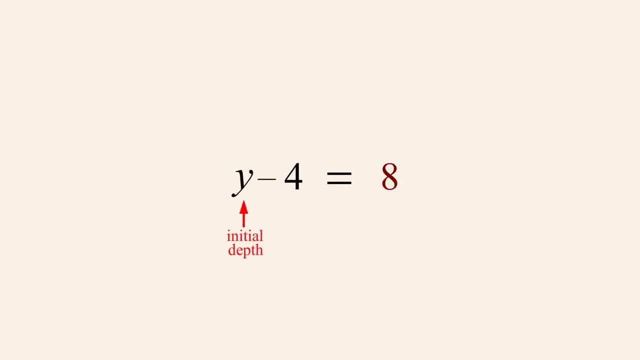 is positive twenty-four thirds or eight. Adding four to both sides of the equation allows us to cancel negative four on the left and negative four on the right and negative four on the left, leaving us with y equals eight plus four or twelve. So the initial depth of the pool when the elapsed time x was zero. 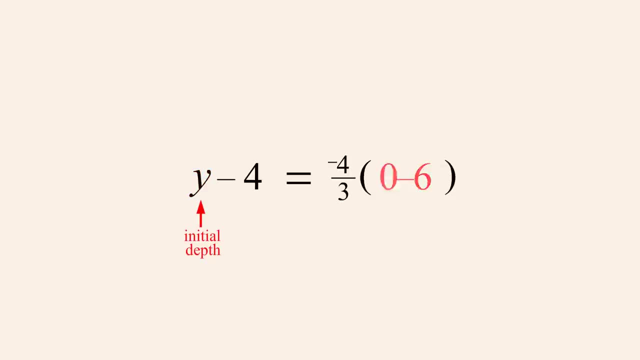 Completing the arithmetic, zero minus six is negative six and negative four thirds times negative six is positive twenty-four thirds or eight. Adding four to both sides of the equation allows us to cancel negative four on the left, leaving us with: y equals eight plus four or twelve. 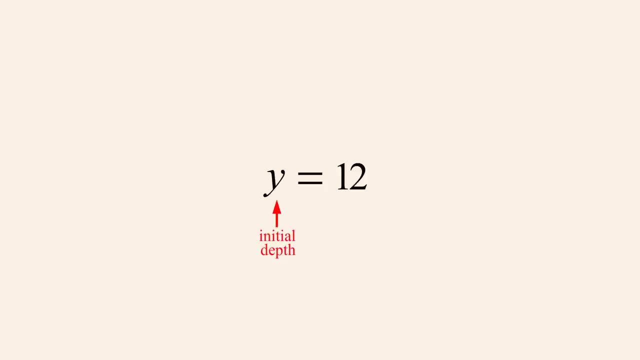 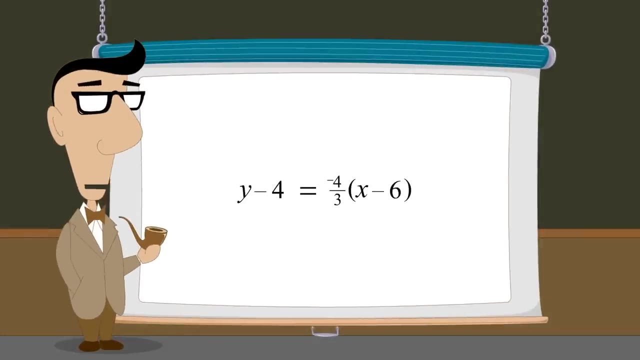 So the initial depth of the pool when the elapsed time x was zero was twelve feet. If we would like to find out how long it will take for the pool to be empty, we can set the water level y to zero and solve the equation for x. 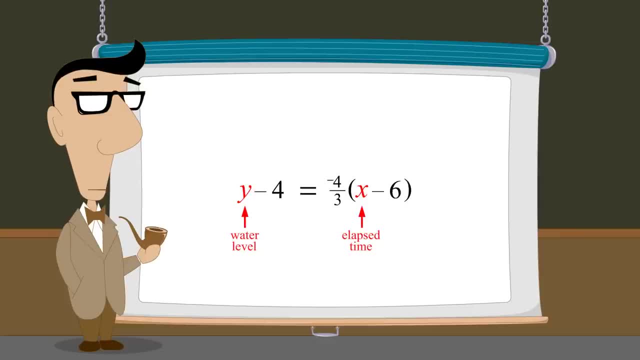 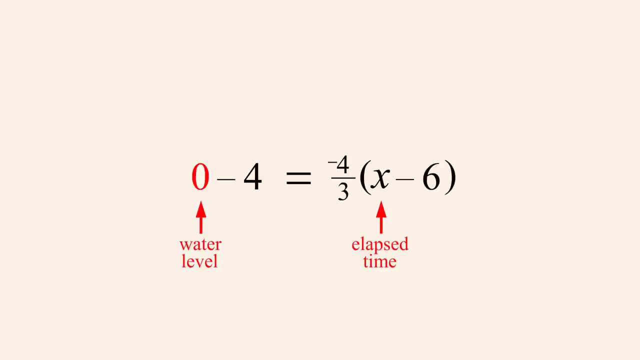 to see what the elapsed time is. at that point We start by setting the value of y to zero, and we can then write zero minus four as negative four. Since we are trying to find the value of x, we want to rearrange the equation so that x is alone on one side. 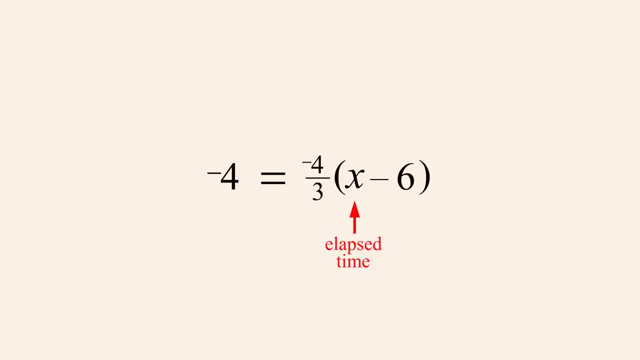 To do this, we must first eliminate the negative four thirds by multiplying both sides of the equation by the reciprocal of negative four thirds, which is negative three fourths, Since anything multiplied by its reciprocal is one. we can replace negative three fourths times negative four thirds with one. 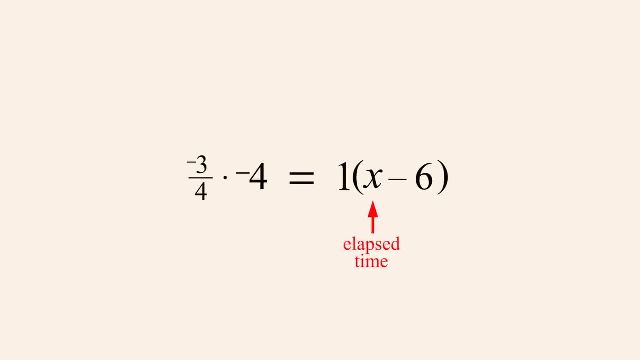 Now, since everything in the parentheses is multiplied by one, we can eliminate the one and the parentheses, Completing the arithmetic on the left side. negative three, fourths times negative four is twelve fourths or three, and adding six to both sides allows us to cancel the negative six on the right. 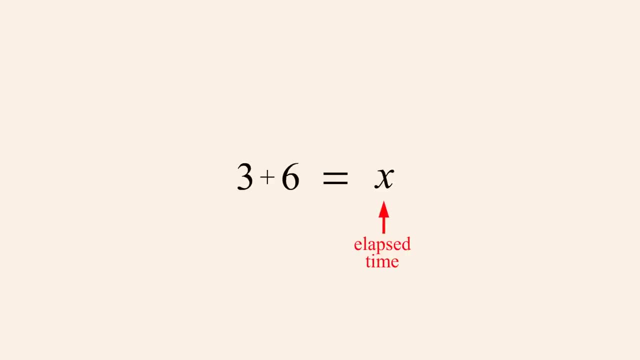 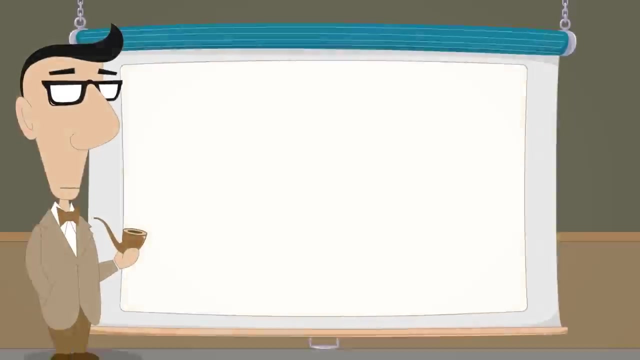 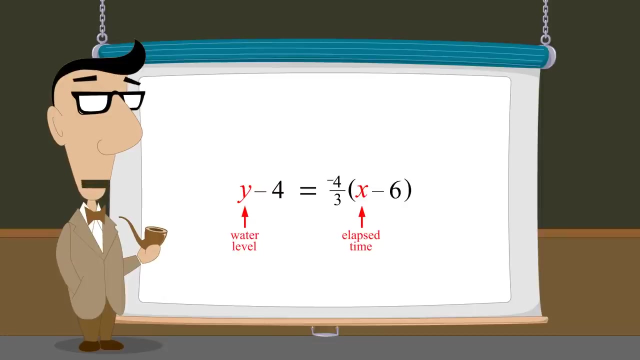 leaving us with the equation: three plus six equals x. Adding three and six, we have nine equals x or, equivalently, x equals nine. So when y is zero, x is nine, Since x is the elapsed time and y is the water level. this result tells us that when the water level y is zero, 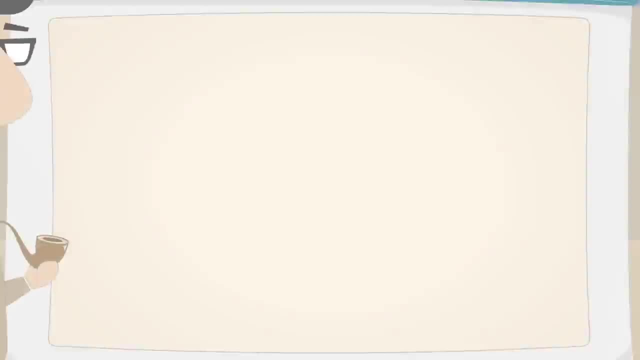 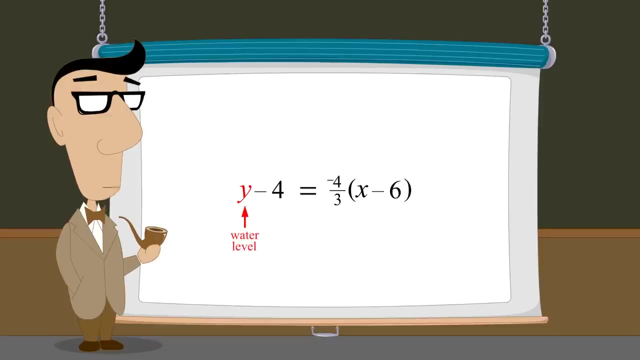 was twelve feet. If we would like to find out how long it will take for the pool to be empty, we can set the water level y to zero and solve the equation for x. to see what the elapsed time is at that point, We start by setting the value of y. 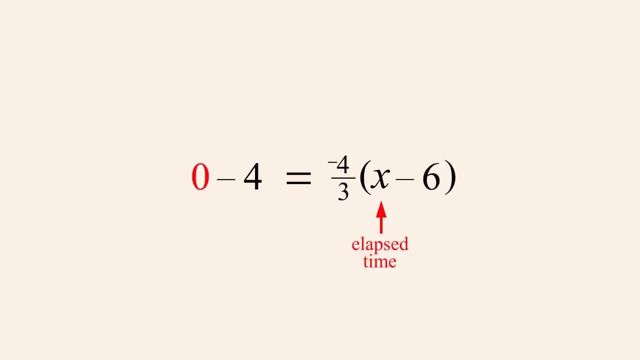 to zero, and we can then write zero minus four as negative four. Since we are trying to find the value of x, we want to rearrange the equation so that x is alone on one side. To do this, we must first eliminate the negative four thirds. 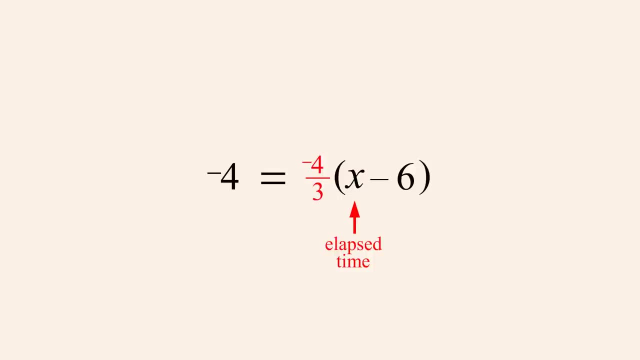 by multiplying both sides of the equation by the reciprocal of negative four thirds, which is negative three fourths, Since anything multiplied by its reciprocal is one, we can replace negative three fourths times negative four thirds with one Now, since everything in the parentheses is multiplied by one. 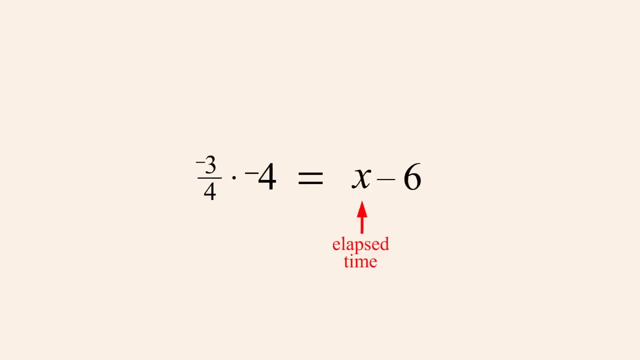 we can eliminate the one and the parentheses. Completing the arithmetic on the left side: negative three fourths times negative four is twelve fourths or three, and adding six to both sides allows us to cancel the negative six on the right, leaving us with the equation: three plus six equals x. 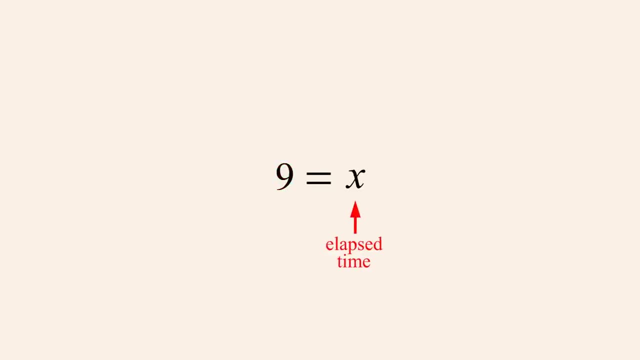 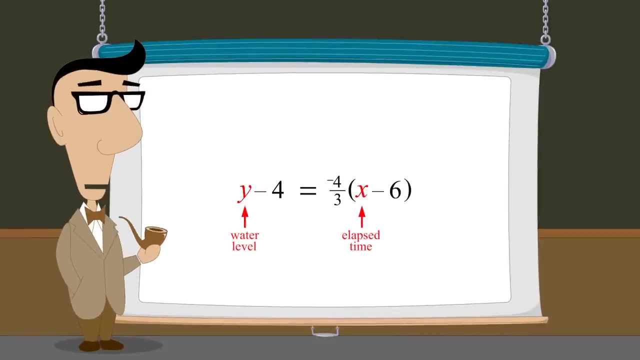 Adding three and six, we have nine equals x or, equivalently, x equals nine. So when y is zero, x is nine, Since x is the elapsed time and y is the water level. this result tells us that when the water level y is zero, the elapsed time x will be nine hours. 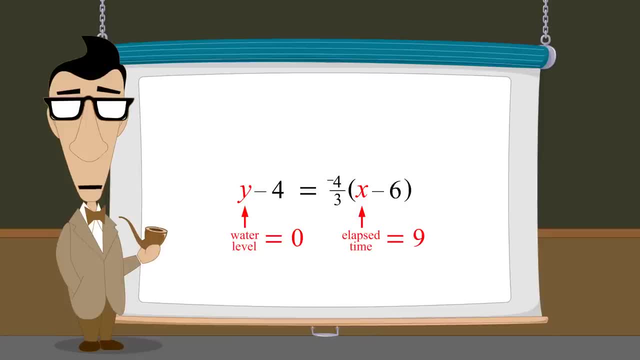 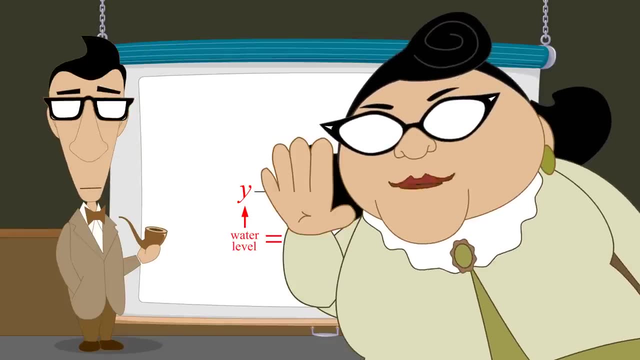 Since the drain was opened at noon, the pool will not be empty until nine o'clock. Excuse me, Professor Von Schmohawk, Did I just hear you say that my pool will not be empty until nine o'clock? Uh, yes, Professor Ethylene. 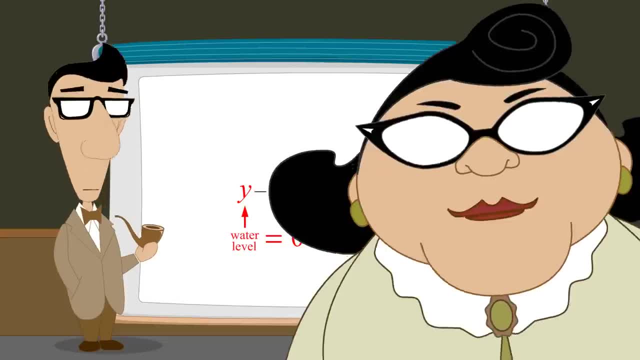 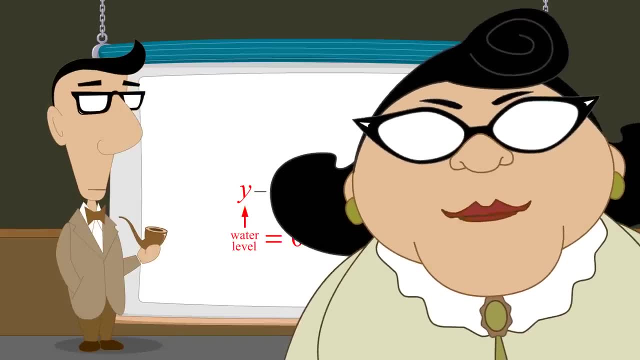 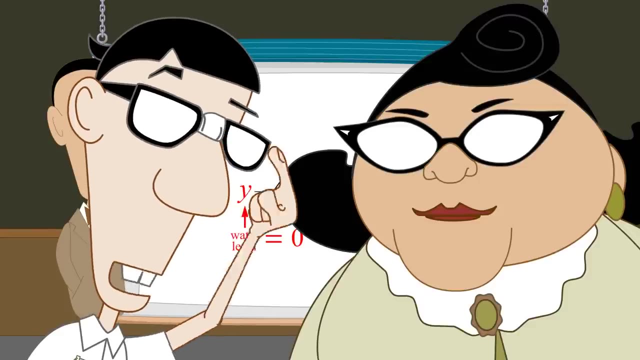 According to our calculations, that is correct, But I distinctly remember telling Mr Moosemasher that my pool must absolutely be empty by the time my guests arrive at eight. Uh, excuse me If I may interject here for a moment. I believe that it is possible to calculate the exact depth of water in your pool. 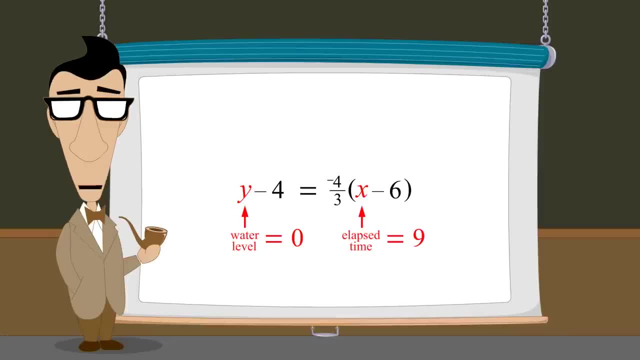 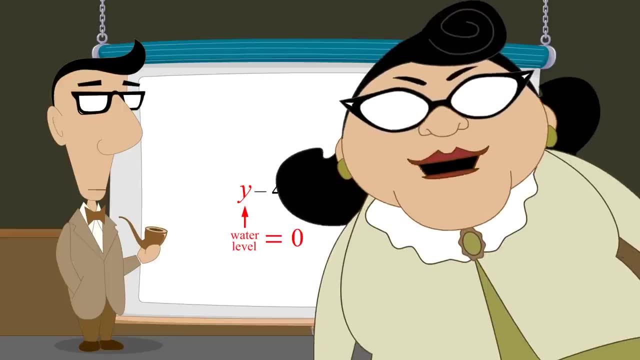 the elapsed time x will be nine hours Since the drain was opened at noon. the pool will not be empty until nine o'clock. Excuse me, Professor Von Schmohawk, Did I just hear you say that my pool will not be empty until nine o'clock? 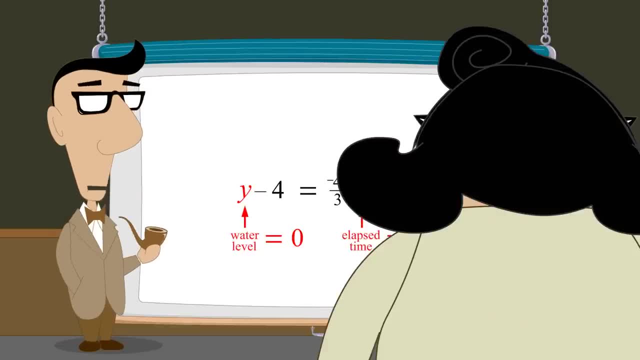 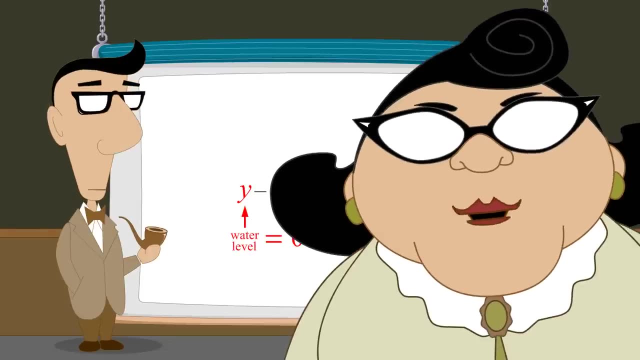 Uh yes, Professor Ethylene, According to our calculations that is correct, But I distinctly remember telling Mr Moosemasher that my pool must absolutely be empty by the time my guests arrive at eight. Uh, excuse me If I may interject here for a moment. 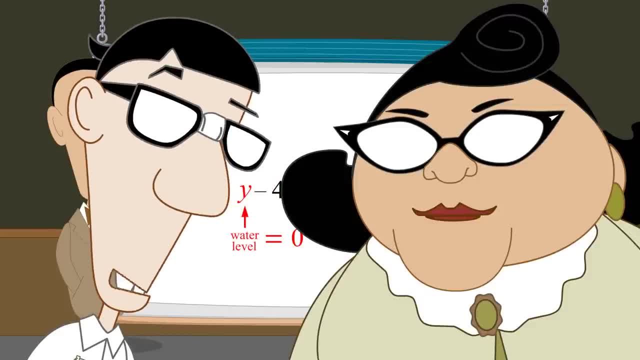 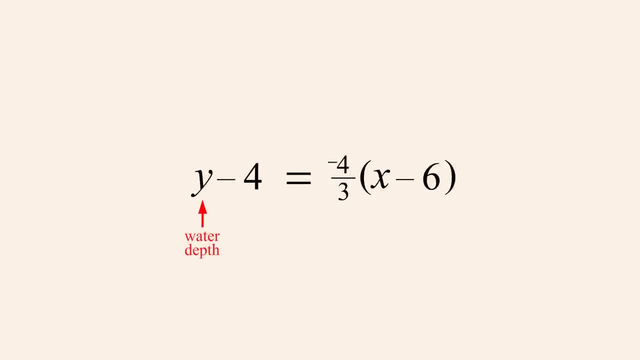 I believe that it is possible to calculate the exact depth of water in your pool at the time your guests will arrive. If we start with the equation for water depth versus elapsed time and set the elapsed time x to eight hours, we can then solve this equation for y. 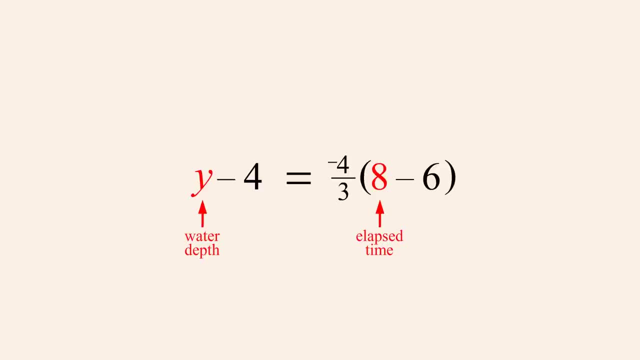 which represents the water depth, and thereby determine the depth at exactly eight o'clock post meridian. As we all know, eight minus six is two and negative four thirds times two is negative eight thirds. Then, adding four to both sides, the fours on the left side cancel. 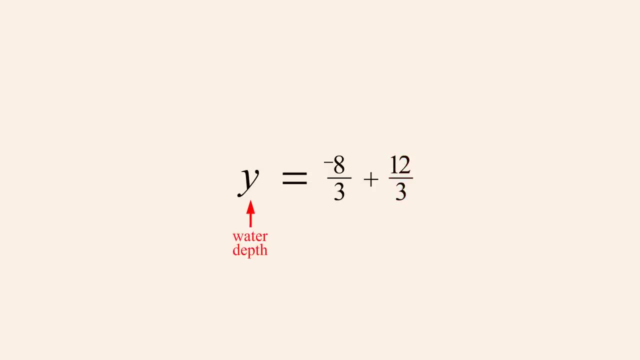 We can then write four as twelve thirds and negative eight thirds plus twelve thirds is four thirds. So according to my calculations, the water depth at eight o'clock pm will be exactly four thirds feet, In other words one and one third feet Now, since there are twelve inches in a foot. 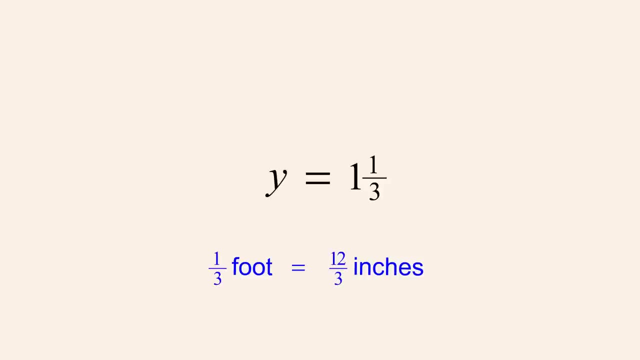 one third of a foot is twelve inches divided by three Or four inches. So one and one third feet is one foot four inches. We can therefore deduce that when your guests arrive, your pool will contain exactly one foot four inches of water. 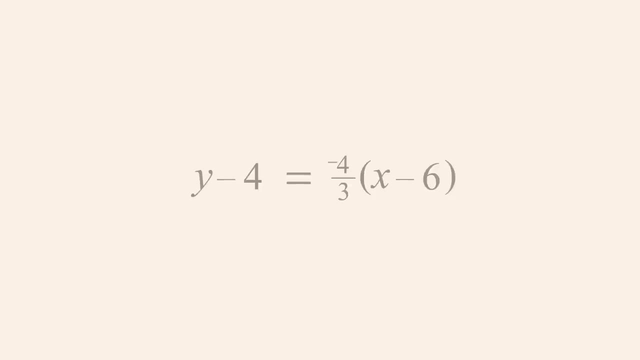 at the time your guests will arrive. If we start with the equation for water depth versus elapsed time and set the elapsed time x to eight hours, we can then solve this equation for y, which represents the water depth, and thereby determine the depth at exactly eight o'clock post-meridian. 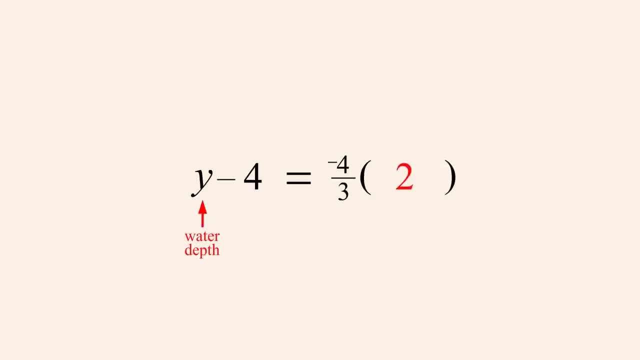 As we all know, eight minus six is two and negative four-thirds times two is negative eight-thirds. Then adding four to both sides, the fours on the left side cancel. We can then write four as twelve-thirds and negative eight-thirds as two-thirds. 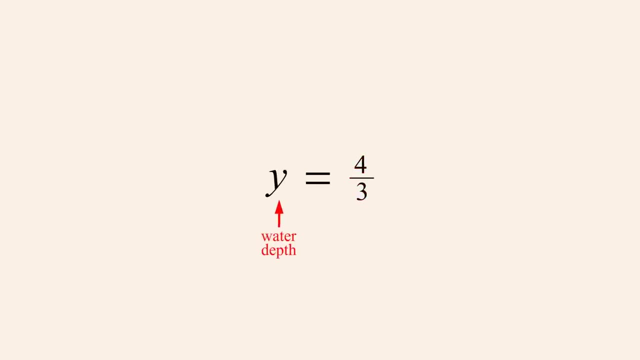 Two-thirds plus twelve-thirds is four-thirds. So according to my calculations, the water depth at eight o'clock pm will be exactly four-thirds feet, In other words one and one-third feet Now, since there are twelve inches in a foot. 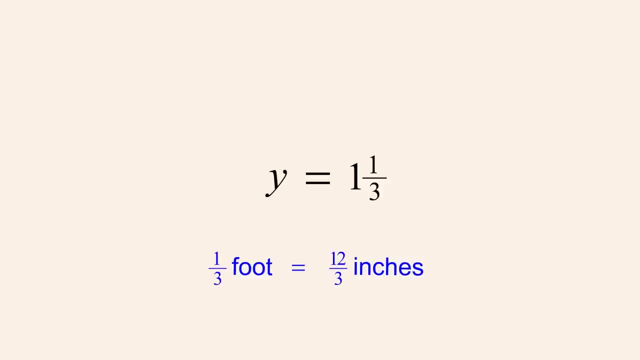 one-third of a foot is twelve inches divided by three or four inches. So one and one-third feet is one foot four inches. We can therefore deduce that when your guests arrive, your pool will contain exactly one foot four inches of water. 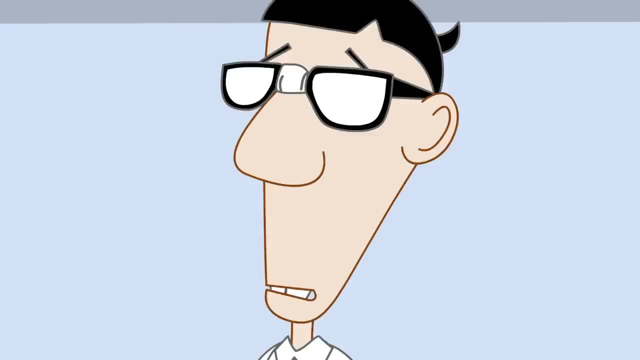 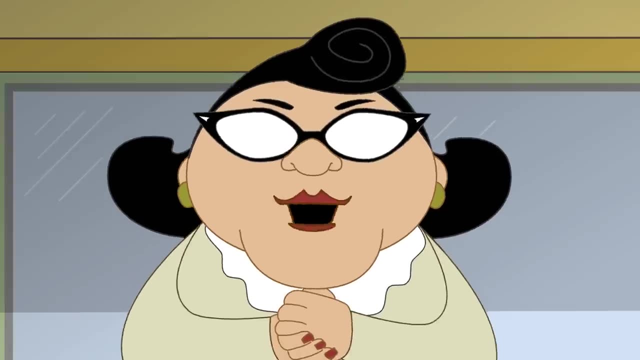 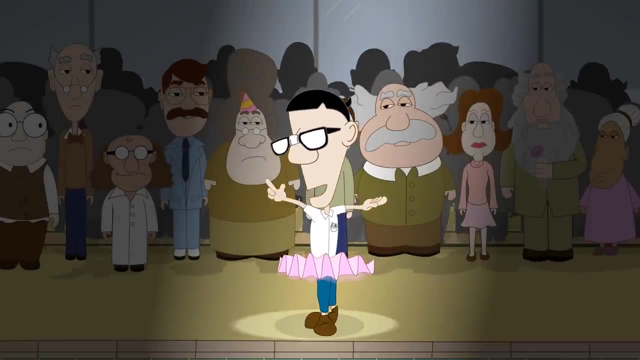 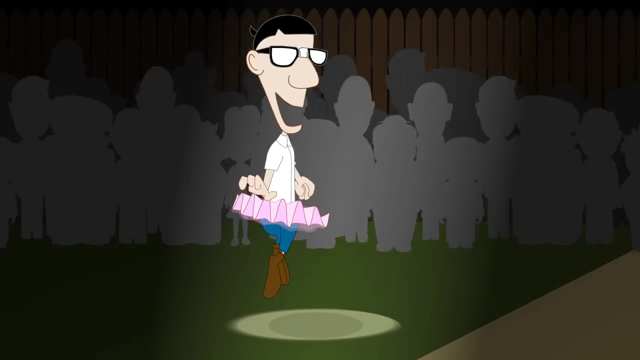 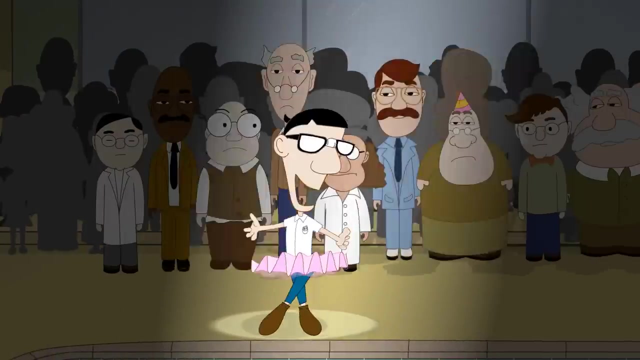 Nope, Uh, Professor Ethelene, how much longer do I have to entertain your guests? Why you're doing a splendid job, AV. I'll let you know when it's nine o'clock. Yeesh, Thank you, AV. 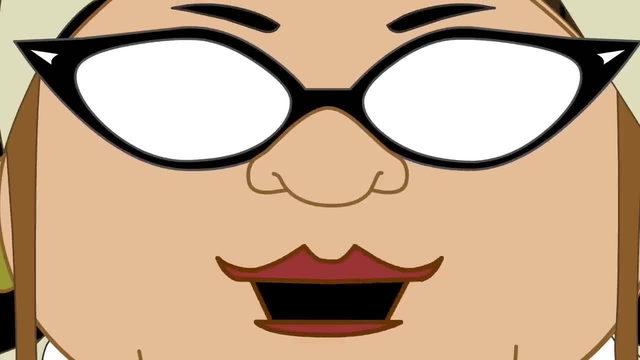 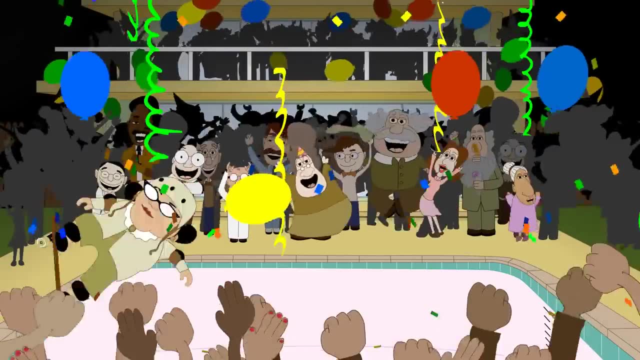 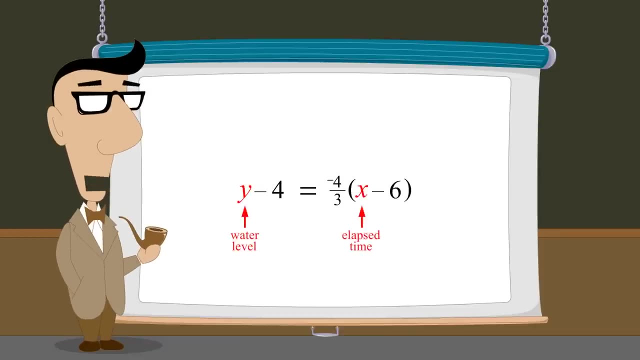 It's exactly nine o'clock and, just as calculated, the pool is empty. Woo-hoo, Oh my Yee-haw. We have seen how linear equations can be applied to real world applications. In the next lecture, we will see how real world quantities can be calculated using formulas. 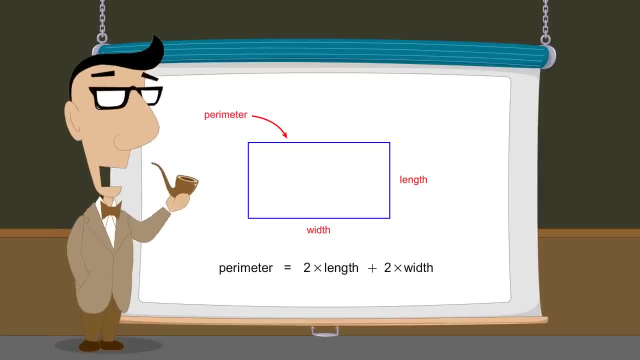 also referred to as literal equations which relate two or more quantities.